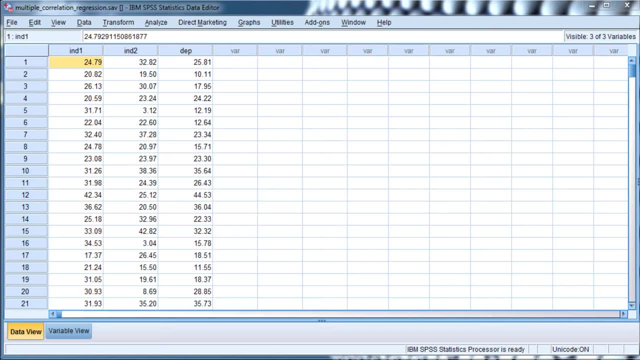 coefficients. but multiple correlation is related to Model R And I'm going to show that multiple correlation is really just a Pearson correlation. So if you understand Pearson correlation then perhaps surprisingly, you also understand multiple correlation. So what I've done is I've 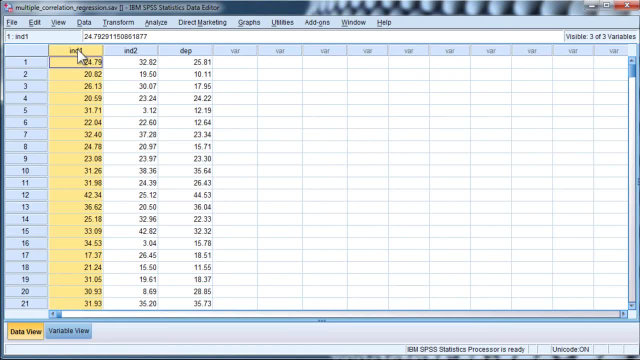 simulated some data to consist of two independent variables and one dependent variable And the purpose of the analysis is to maximally predict the dependent variable based on a combination of independent variable one and two. So I'm going to analyze regression and linear and I'm going 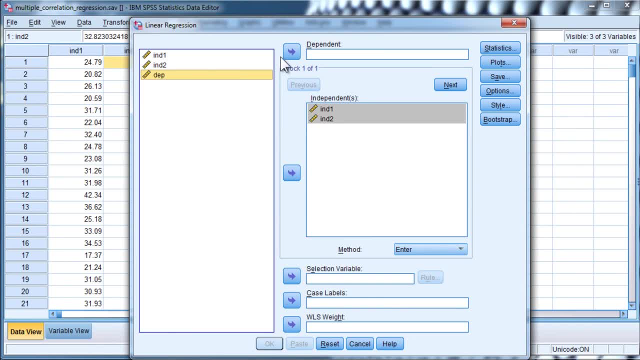 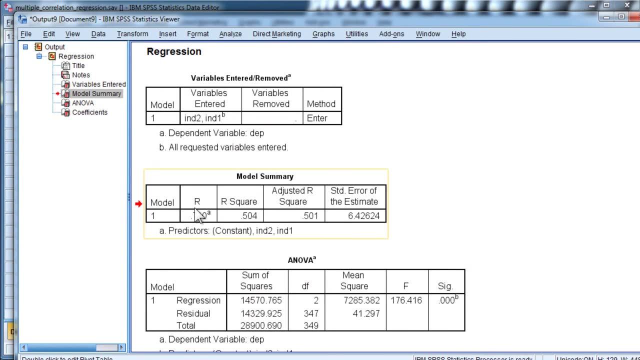 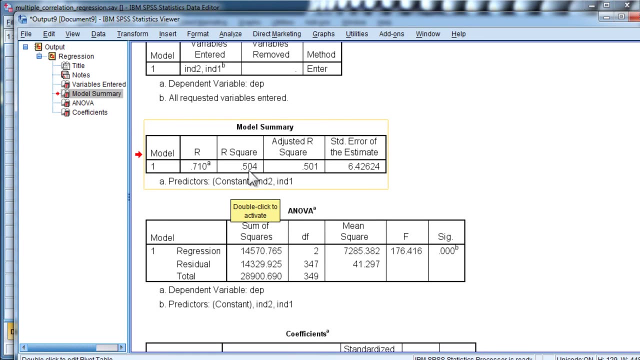 to include the two independent variables in the independent variable. And then I'm going to include the two independent variables in the independent variable, And then I'm going to click OK And here are the results. So the Model R comes out to 0.710, which implies that 50% or 50.4%. 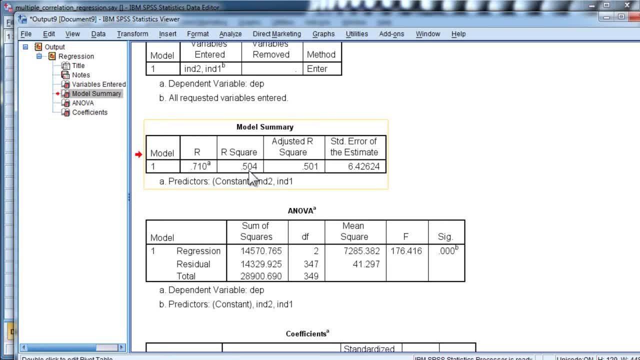 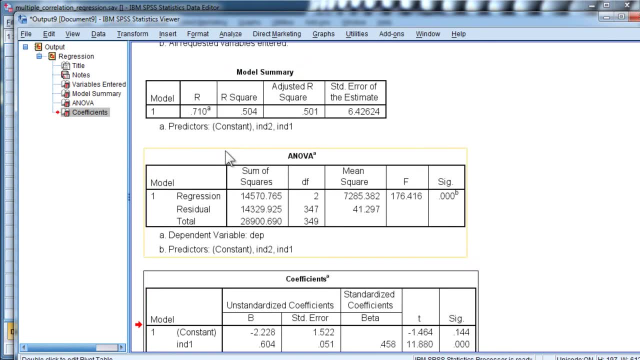 of the variance in the dependent variable was accounted for by the combination of the independent variables, And this is statistically significant. Now, how does this value of 0.71 come about? What is that? Well, it's a combination, yes, of the two independent variables created to maximally. 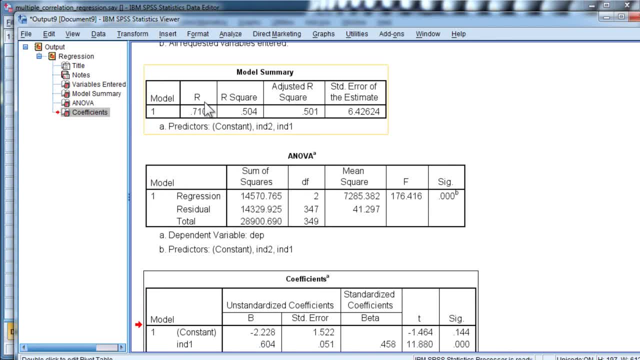 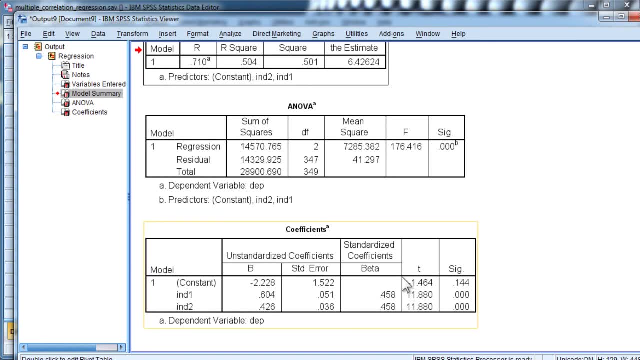 predict the dependent variable. But in very real terms, this multiple R is simply a Pearson correlation And I'm going to prove it to you. I'm going to prove it to you a little bit the long way, showing you how these beta weights correspond to the multiple R, even. 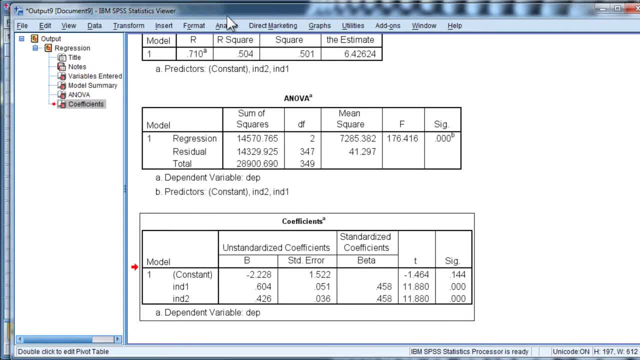 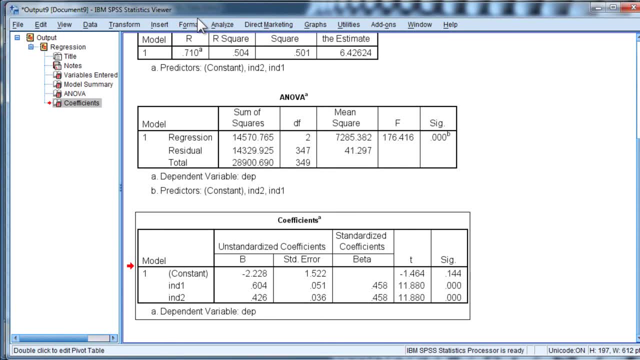 though this is really the multiple regression. So, in order to show that multiple R is just a Pearson R, what I need to do is I need to create prediction. I need to create an iterative prediction. I can use my gotto method to generate predictions. 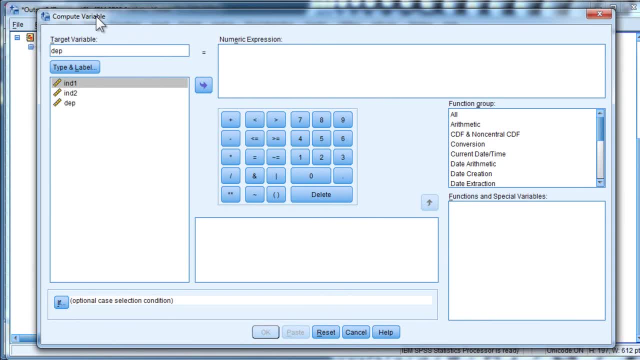 so that I can run the model. There are two ways I can think of to do that. I'm going to do it a little bit the long way, just to show you the inherent, just to understand multiple regression better. So dependent predicted And the way that you would predict the dependent. 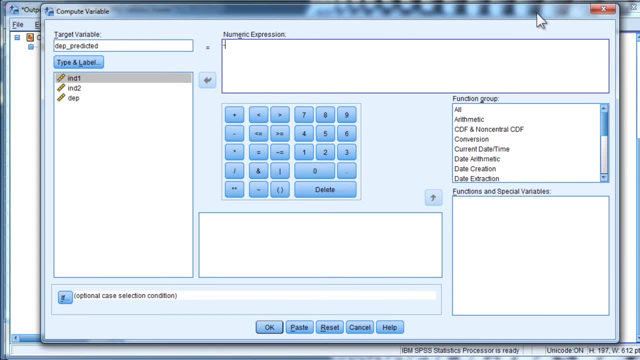 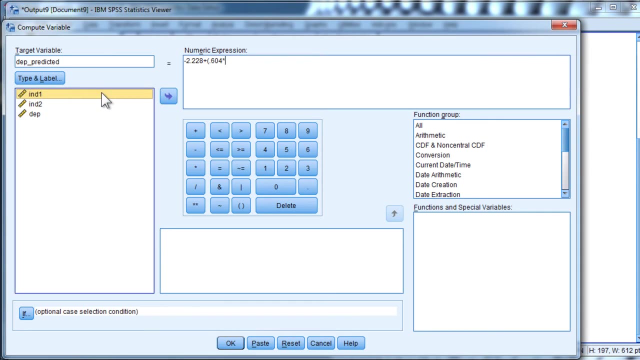 variable is by using the regression equation, which has an intercept of negative 2.28, and unstandardized beta weights equal to 0.604.. I need to multiply that by this independent variable. I'll assume that you already understand the regression equation in multiple regression. 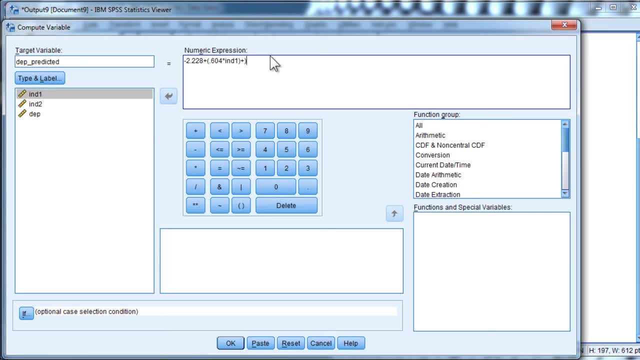 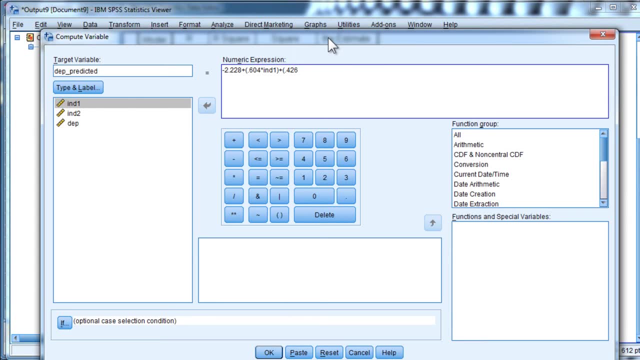 and then I need to add the second predictor, 0.426 times independent variable 2.. So this is the multiple regression equation in the unstandardized form. I've got the intercept negative 2.228, plus the product of the 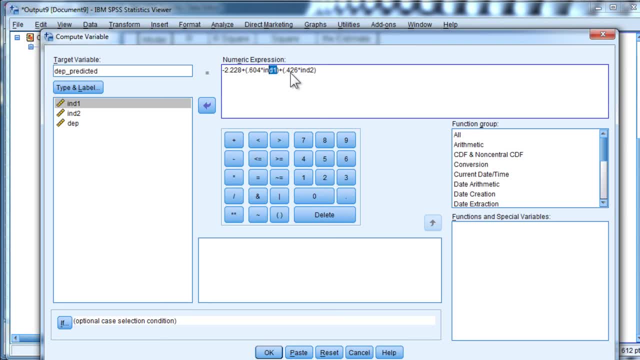 unstandardized slope for independent variable 1, which is multiplied by the independent variable 1 case values. and then I'm doing the same thing with independent variable 2, multiplying independent variable 2 values by the unstandardized slope for independent variable 1.. 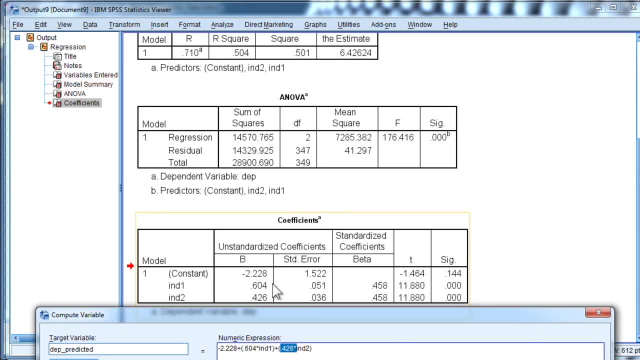 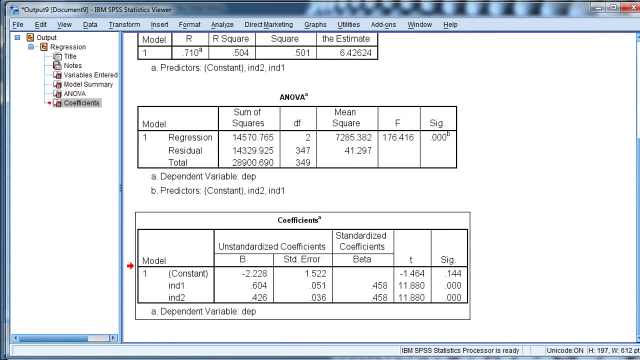 unstandardized slope. So that's where those values come from: Negative 2.228 plus 0.604 multiplied by independent 1, etc. And this is going to create predicted values. dependent variable predicted values. Click on OK and SPSS. 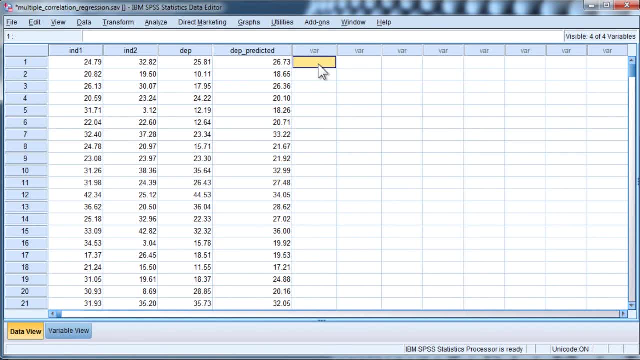 will have created a variable called dependent variable predicted. Now, if you look at the dependent variable and dependent variable predicted, you'll see that the scores are to some degree similar. And the question is well, how similar are they? This multiple regression created a regression equation. How good is it at predicting? 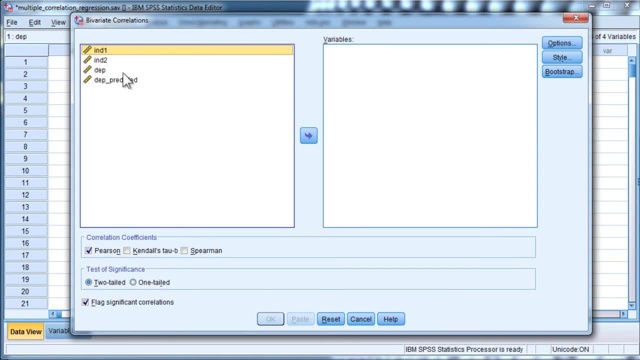 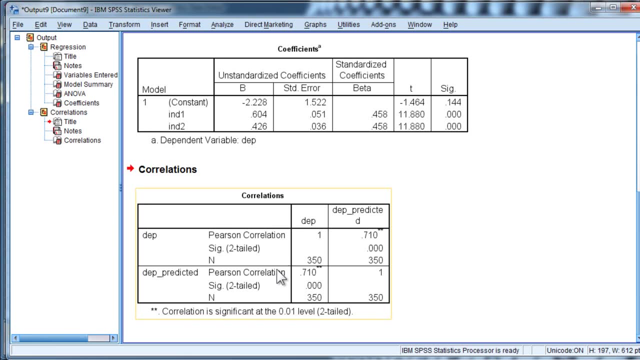 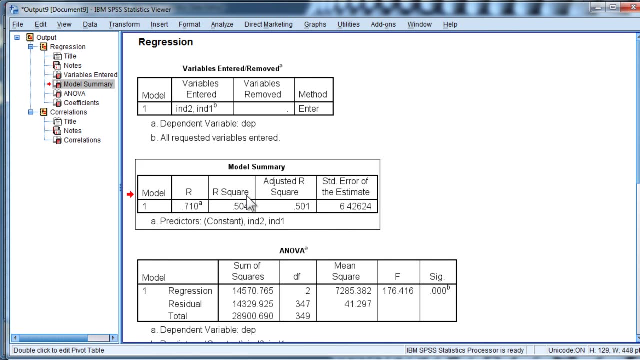 the actual dependent variables. Well, I can estimate that by calculating a correlation between the dependent variable and the predicted dependent variable, and I get exactly 0.710, which is exactly the same thing that you would get from the model summary. So to me when I was learning, 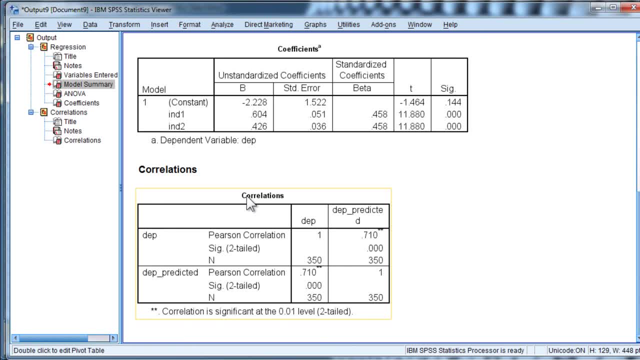 statistics. this was insightful to me to know that the multiple correlation in the context of multiple regression is really just a Pearson correlation. It's a Pearson correlation between the predicted values determined by the regression equation and the dependent variable values. Now, what's also interesting about creating?